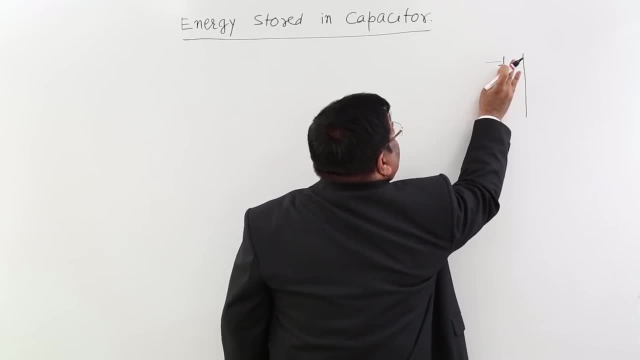 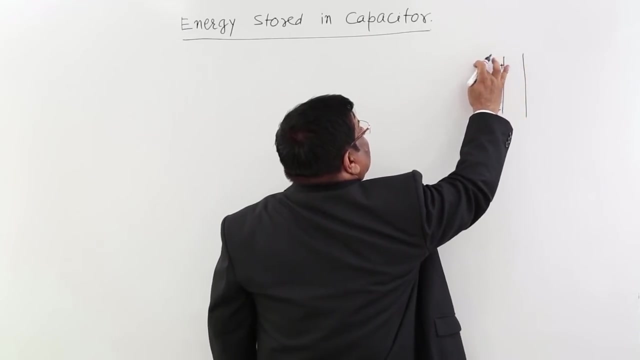 When I want to give it next positive charge, this plus will repel. So I have to apply a force, do the displacement and do the work Similarly, this force will go on increasing when the charges are increasing and finally, I have to do lot of work to keep them here. 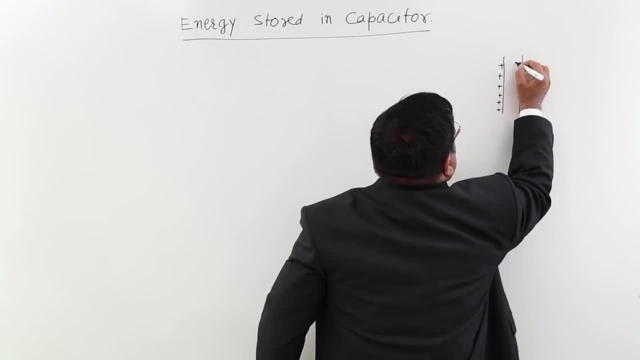 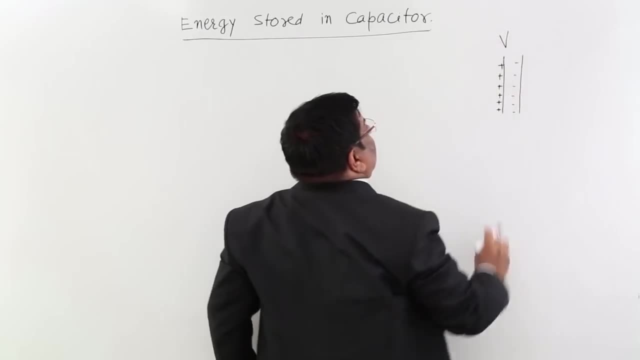 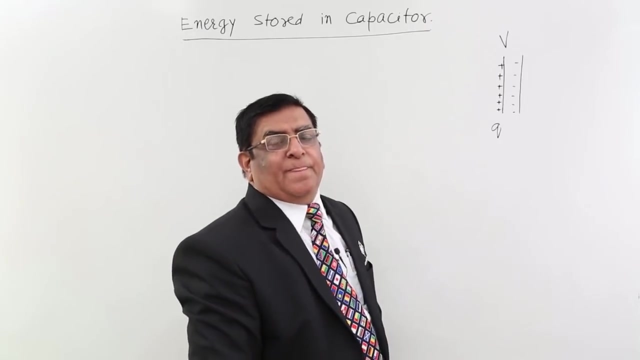 Okay. So this plate, of course with induction. there will be negative here. Okay, By giving the charge the potential rise to V, and the charge stored here is Q. Now, how do I calculate work done? The answer is in electricity. whenever you have to calculate, 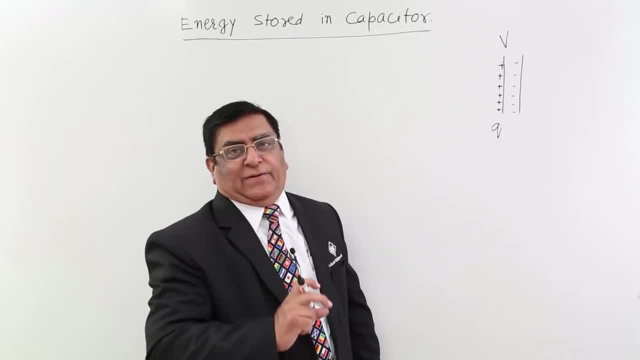 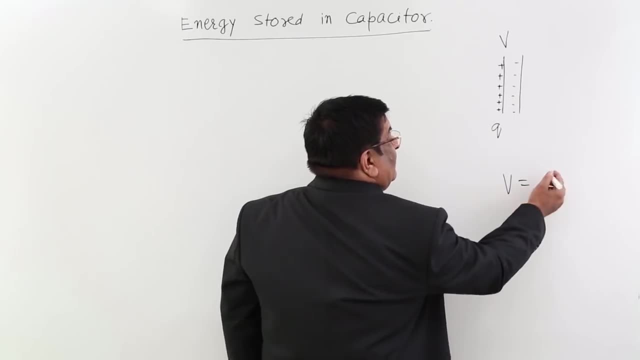 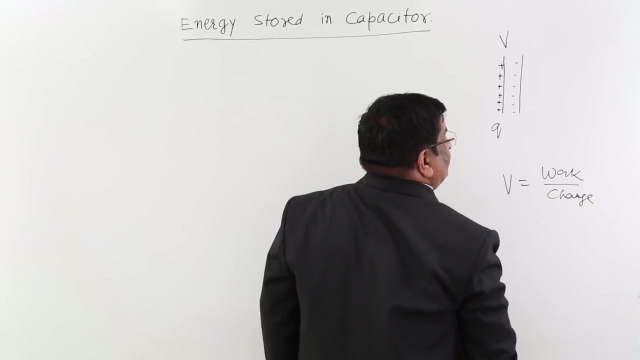 work done. you have to do it with potential, because potential, initially we made this concept of potential by the formula work done on a unit, charge Okay, Work upon charge Okay. And this work is what? Force into displacement, Force into displacement. 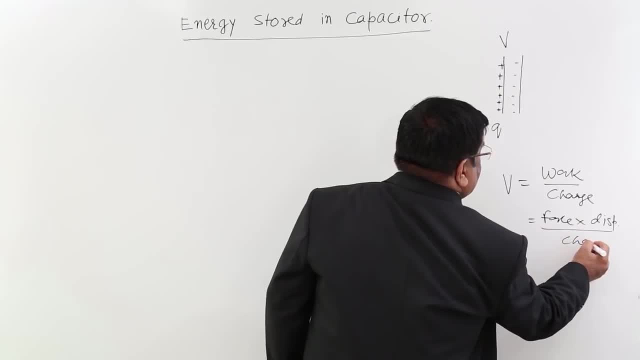 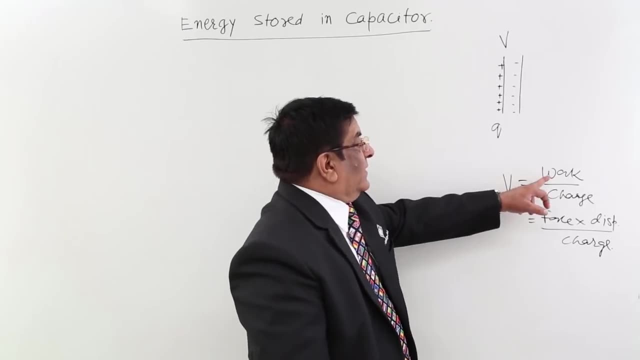 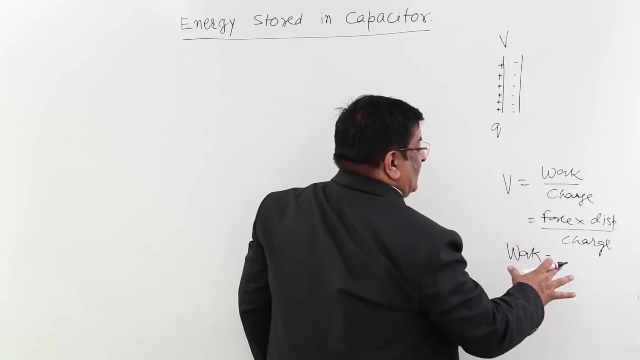 charge. Okay, So this is potential related to work. So work is equal to what Potential into charge? These are the different formulas, These are the different formulas, mechanics, we all know. So here work W is equal to Q. 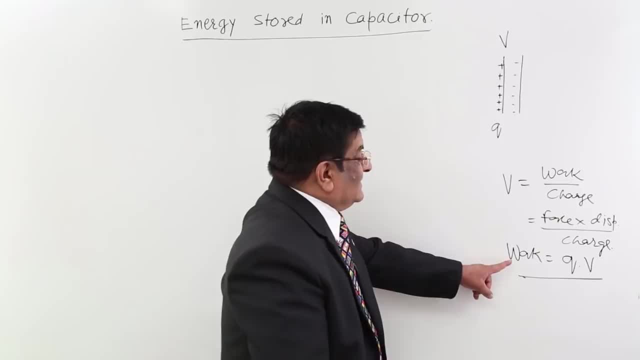 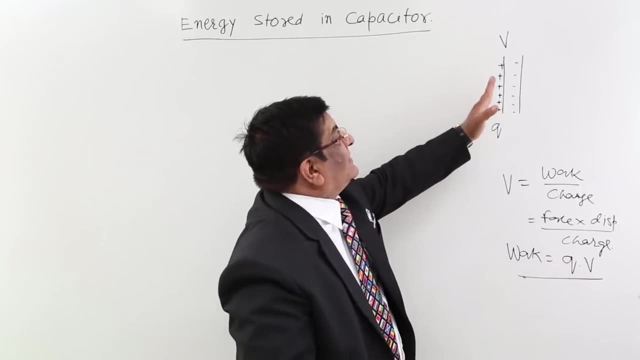 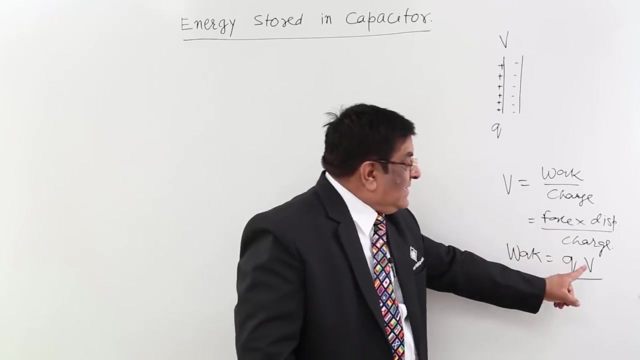 into V. But the thing is that when we started working the potential was 0. When we put certain charge, potential increased. Again we put certain charge potential increased. So finally it has come to this value. So initially, how much work we did Initially. 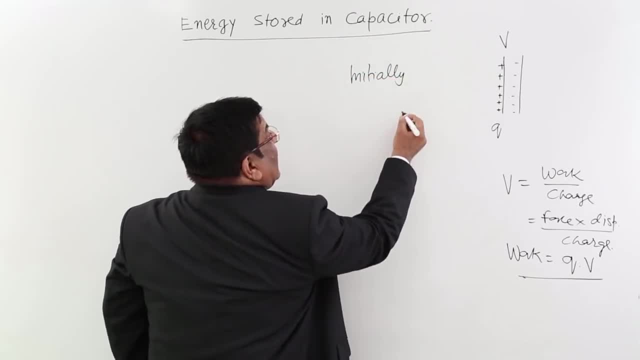 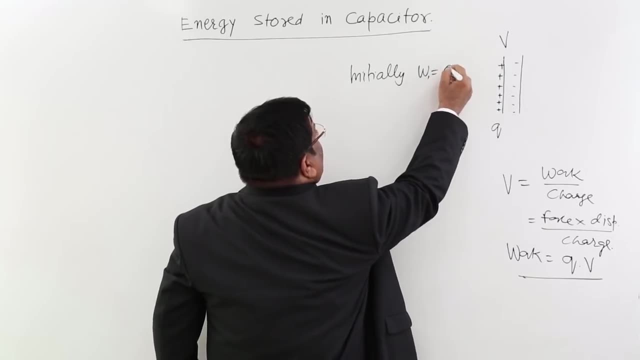 we had to do work. when we were putting first charge, We had to do work 0.. Finally, when I put the last of this charge, Q, the potential had gone to V. How much work I had to do? Final Q into V. This is initial, This is final. So what is the potential We have to calculate? 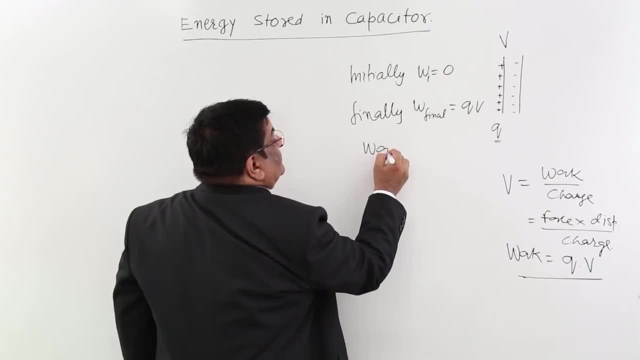 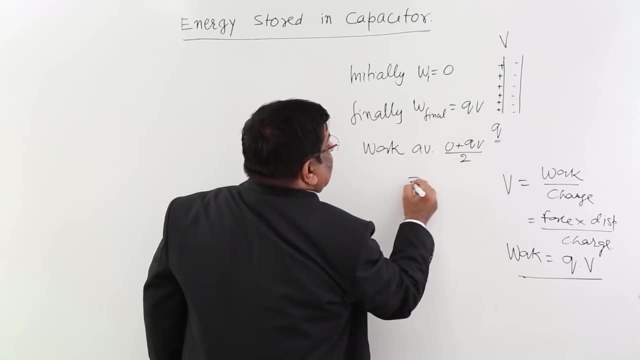 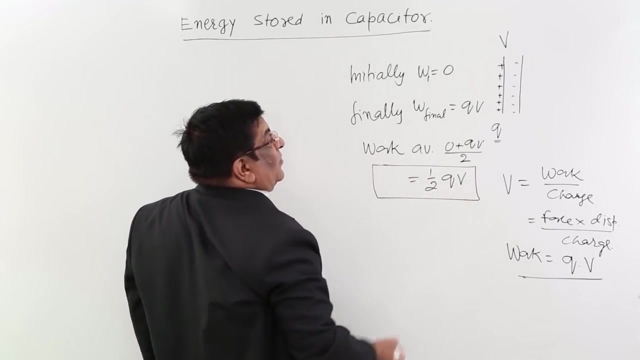 What is the average work done? Work average: This is 0 plus Qv upon 2. This is half Qv. This is the average work done for the full value of v. So this value of v, which was 0 initially, 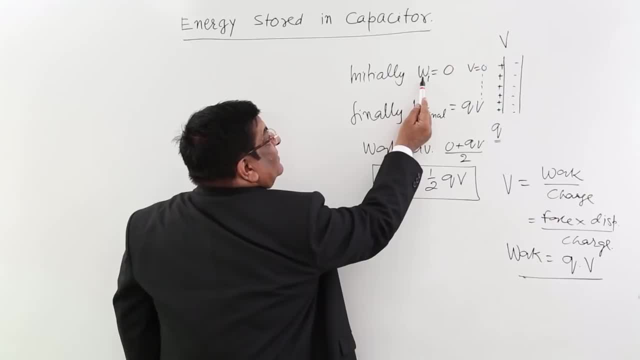 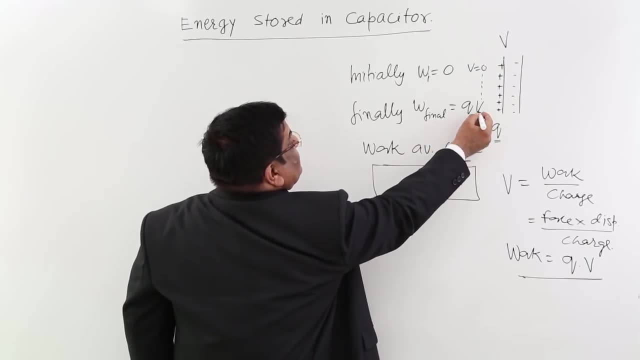 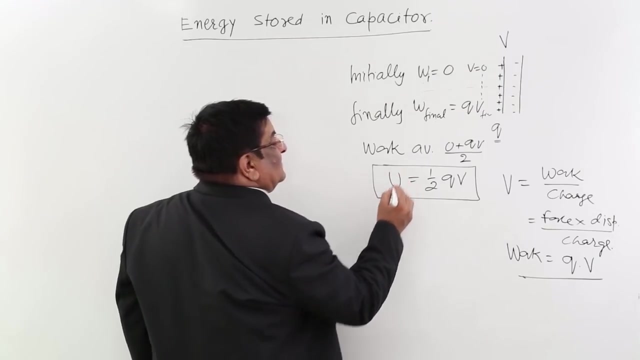 increase, increase, increase. Every time I was doing w2, w3, w4 and final w was Q into v. This is the final v. So initial work done- 0,. final work done- Q- and what will be the average work done? That will be half Q into v. This is energy. This appears to be a very 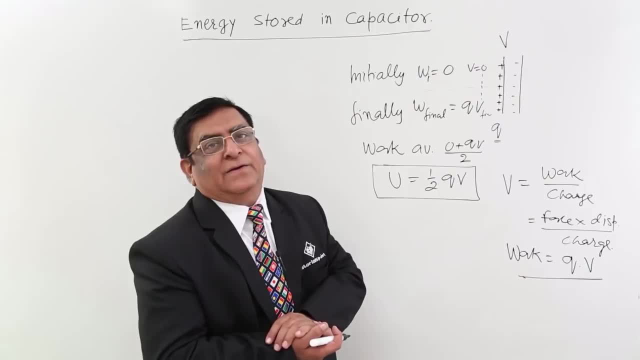 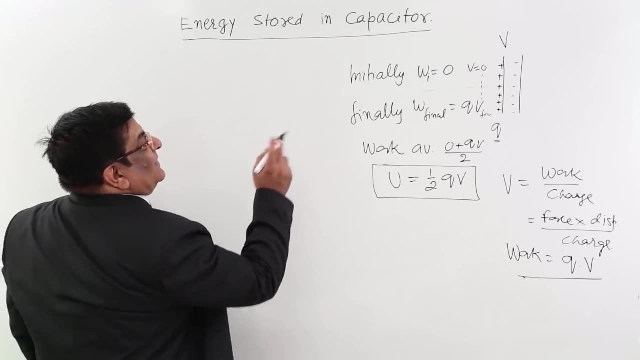 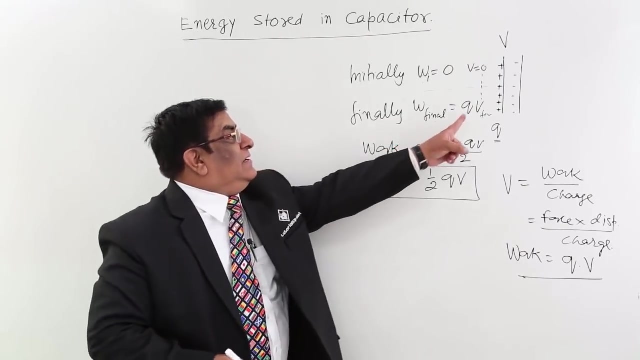 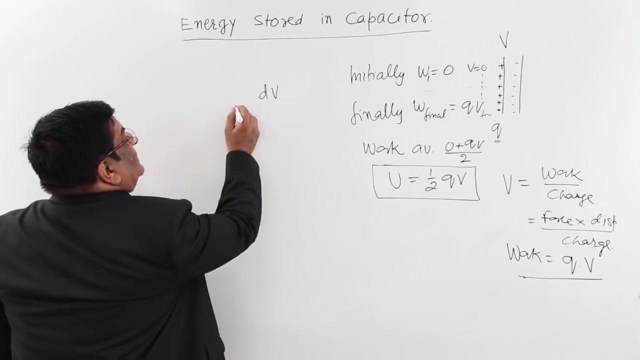 simple method. So some teachers do not agree. They say, let us complicate it. So how do we complicate it? Suppose I give it a very small, I give it a charge Q. With that there is a small change in v- dv. Then the work done is Q into dv. 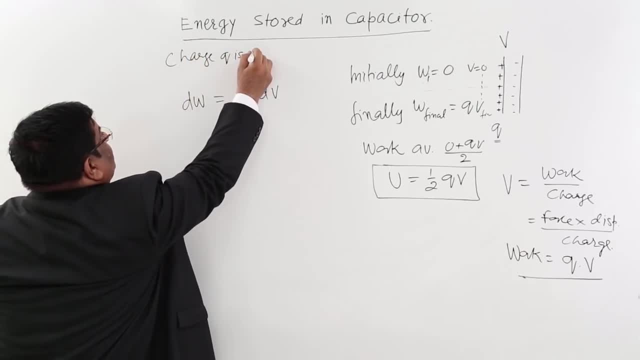 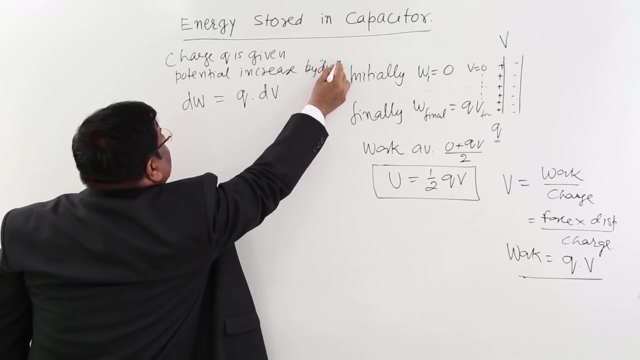 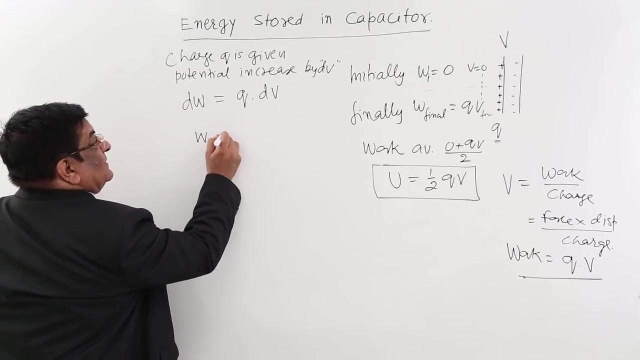 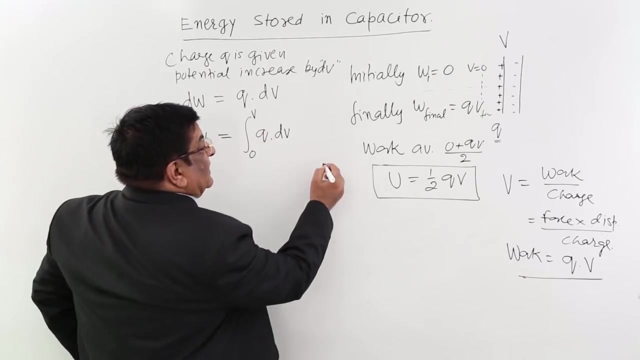 Charge Q is given Potential increase by dv, Then what is the small work? dw is equal to Q into dv. And now what is the total work done? when we increase the voltage from 0 to v, Then this will be integration of Q dv. For each small dv, if I have increased v is: 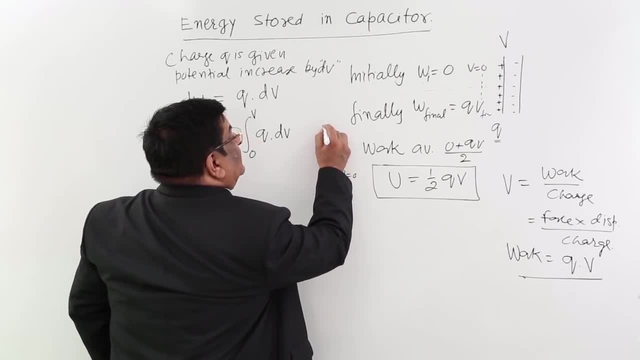 equal to 0. to this height, which is v, is equal to v. So this I have divided into dv, dv, dv, dv. I give the charge, Q raise potential, dv. How much work is done? Q into dv. Q into dv. 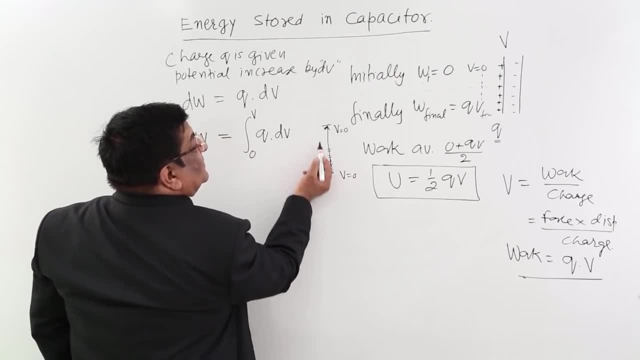 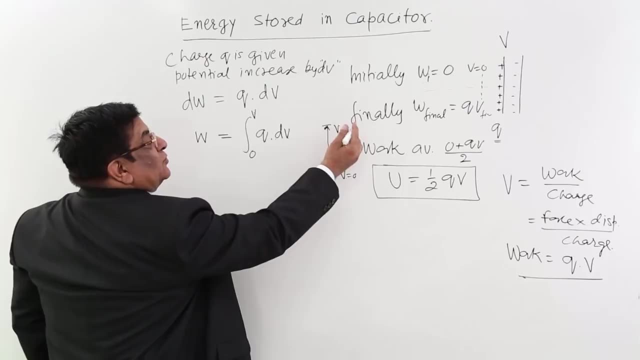 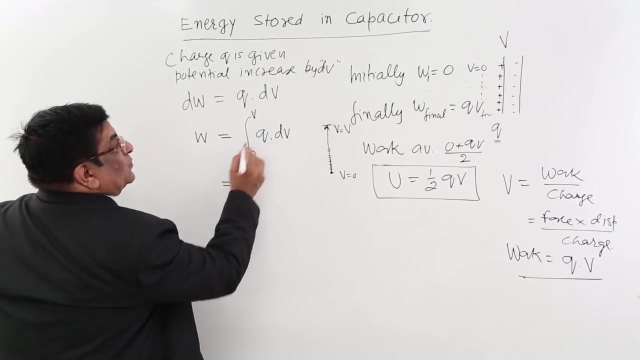 Q into dv And the total work from this to this is integration Q into dv and this integration I will do from v is equal to 0 to v is equal to v. So this is mathematical method. Now this Q, we know by the formula Q is equal to C, into 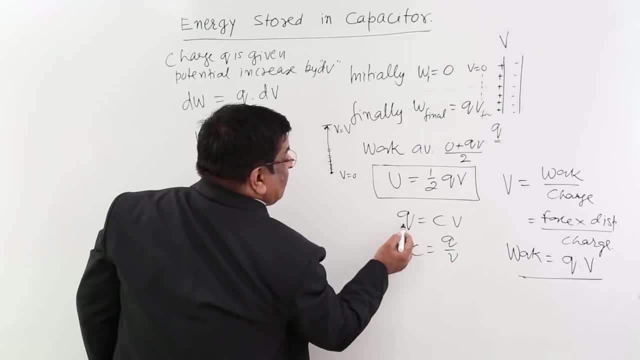 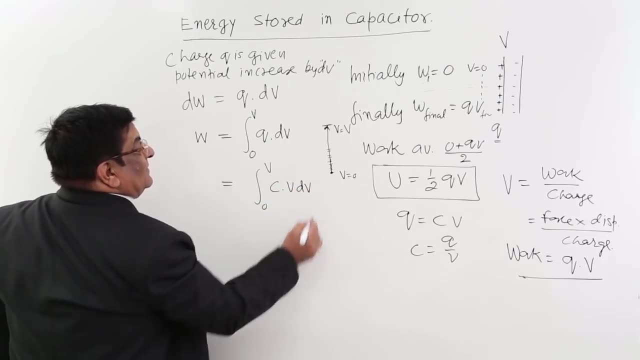 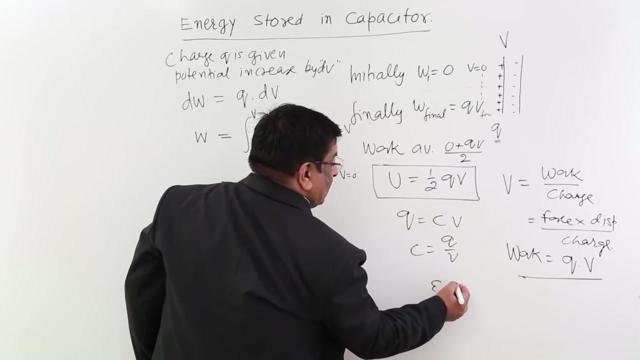 v, C is equal to Q upon V. From this we get: Q is equal to C, v, So I put it as 0 to v, C, V, dV. Now, C is capacitance, which depends upon epsilon0 A upon D During this charging. 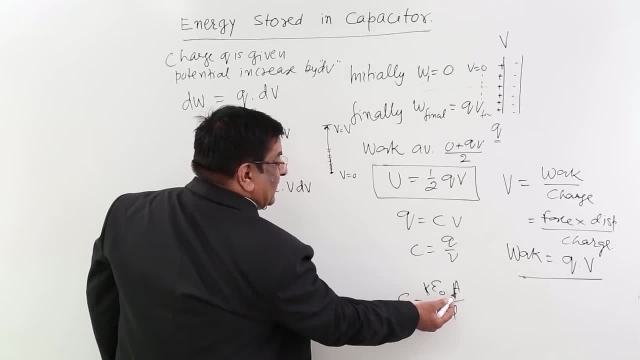 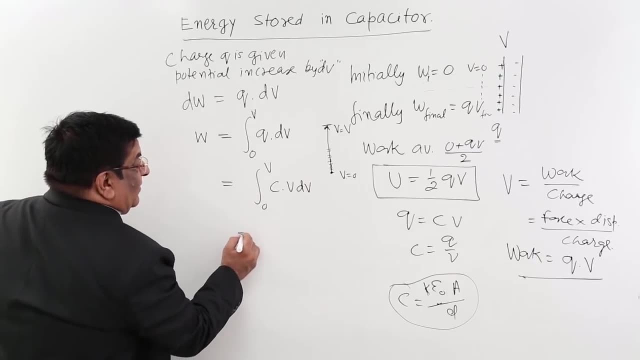 process. neither K change nor epsilon change, nor A change, nor D is changing. So this remain a constant. C remain a constant. it will come out. Integration of V- dV is V square upon 2.. So this is half C V square. This is work done, and this work done converts to energy. 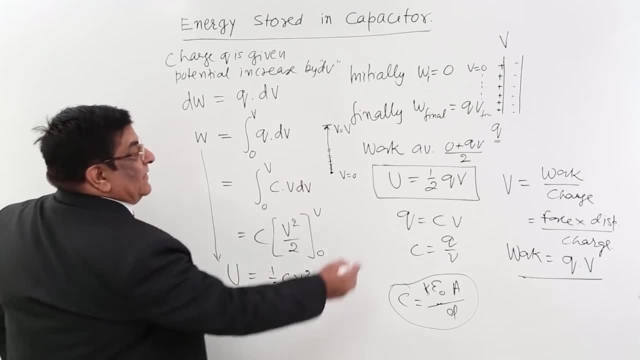 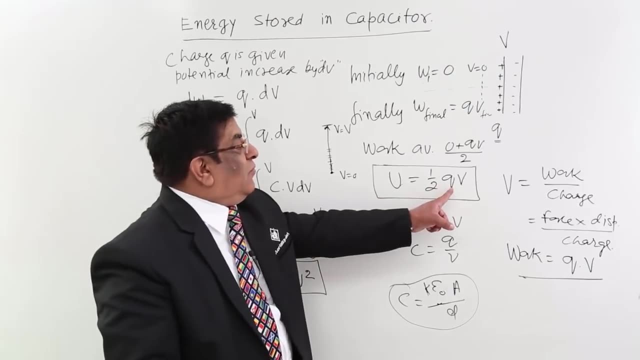 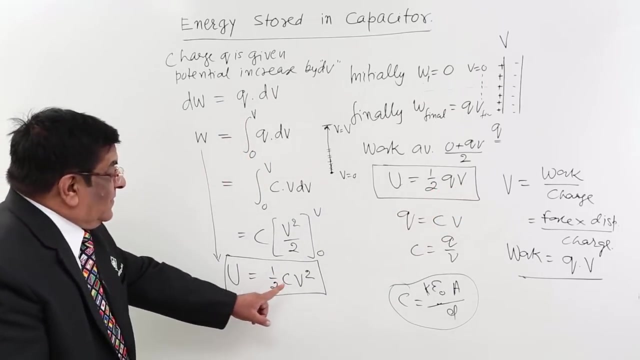 So energy is half C V square We did energy is equal to half Q V. So these two formulas and Q is equal to what C into V. Put it here What it will be: Half C V, Half C V. square Here one C and one V make it Q, So that will be Q into V. So both are. 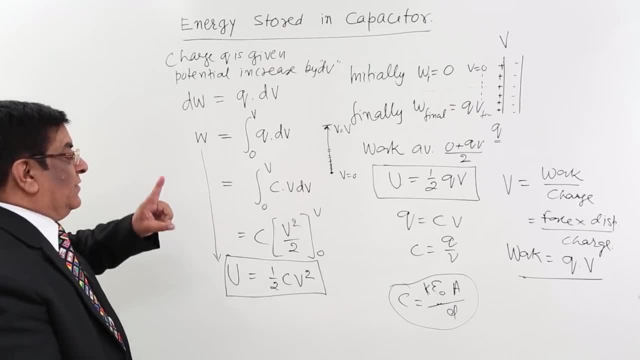 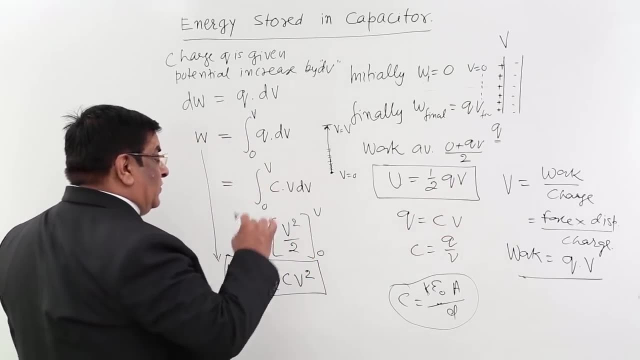 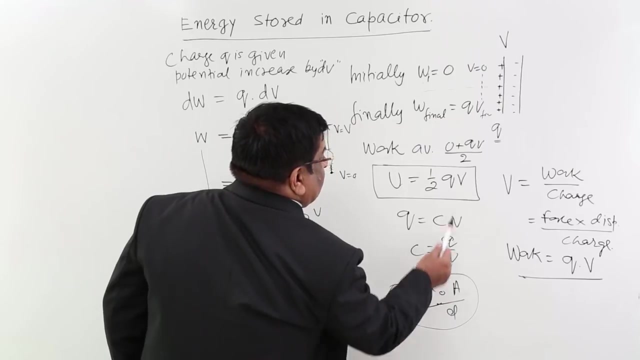 same formulas. We can even convert it into a third formula. This is C into V, This is Q into V, and one we can have Q and C. How This V is equal to Q upon C. Put it Q upon C here. 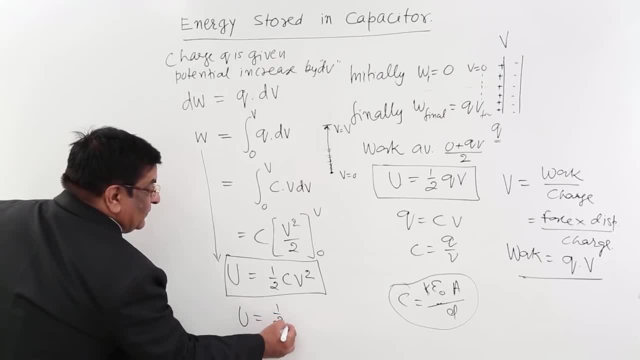 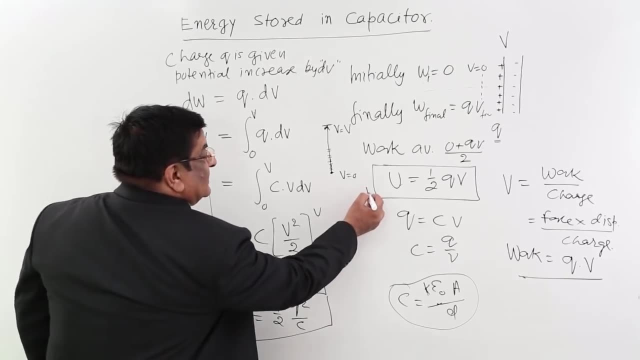 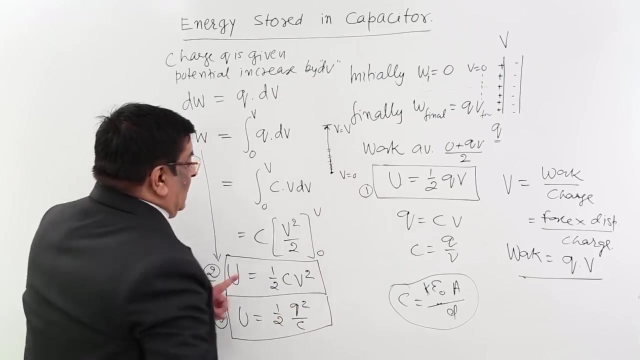 So this will be: U is equal to 1.. U is equal to half Q square upon C. This is third formula. So this is one form, This is other form, This is third form. These are the three formulas for energy given to a capacitor. 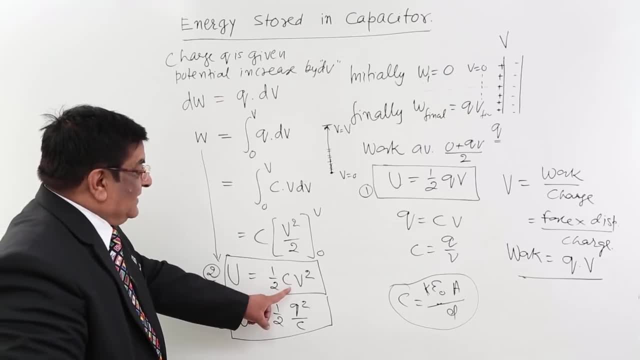 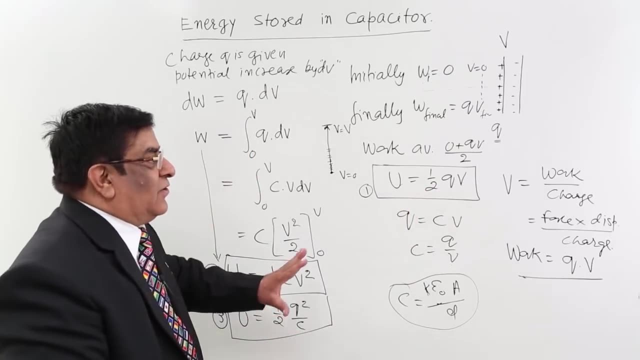 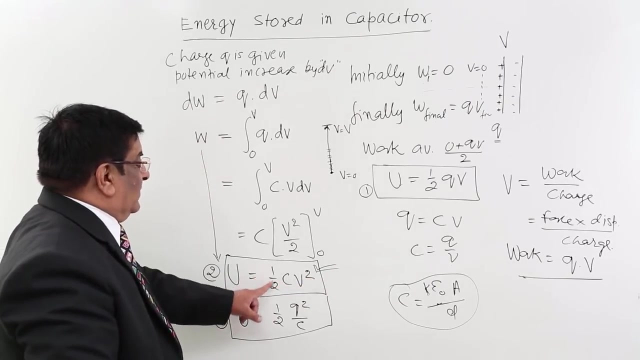 Most of the time we are using this formula because C is a measurable quantity, V is a measurable quantity, Q and Q: These are not measurable quantity. Q and Q, These are not measurable quantities. so this is more acceptable and measurable formula. u is equal to half.